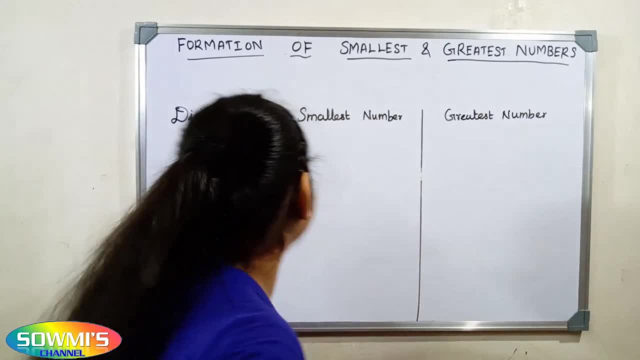 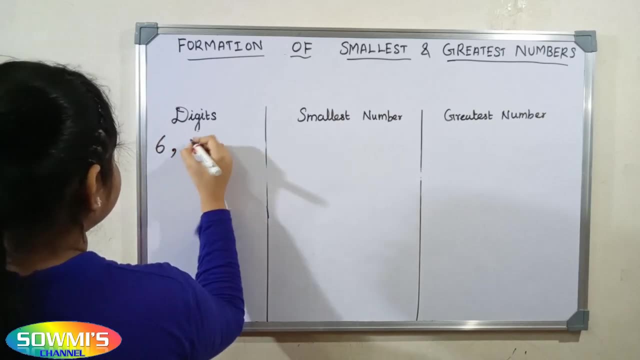 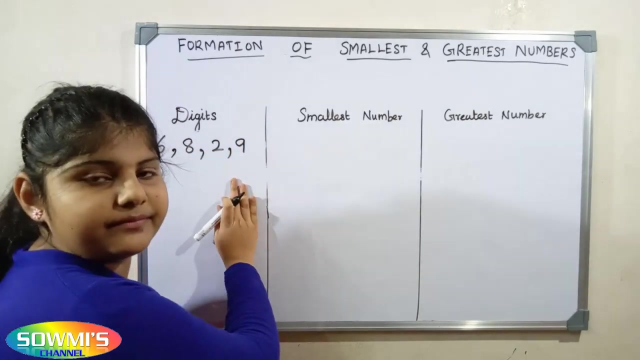 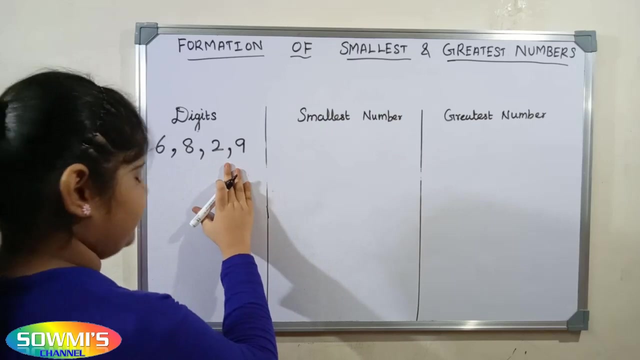 videos regularly. Come on, let's go to the video. For example, we can take 6,, 8,, 2, 9.. First we will form smallest number. To form smallest number now, we have to arrange these digits in ascending order. Ascending order means arranging the digits from smallest number. 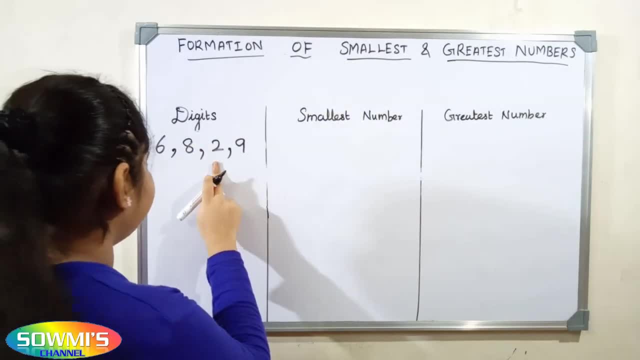 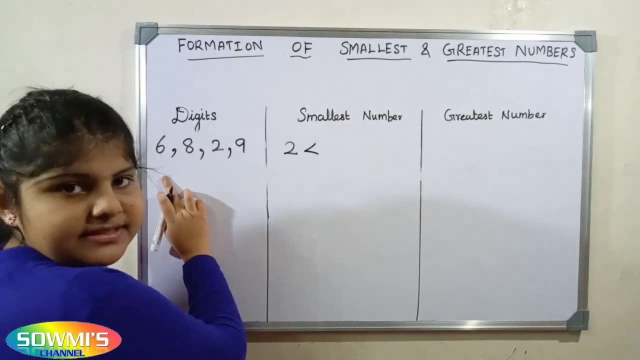 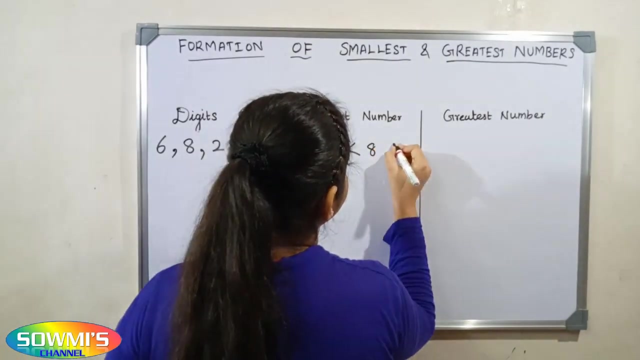 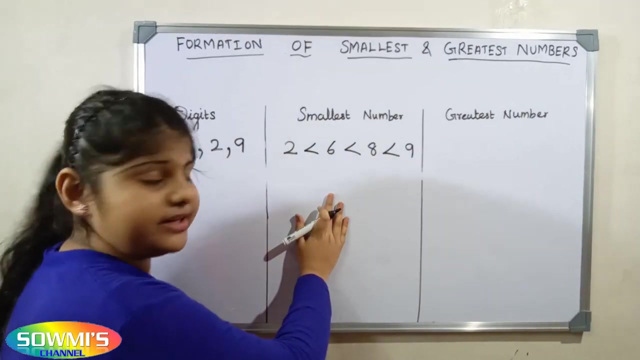 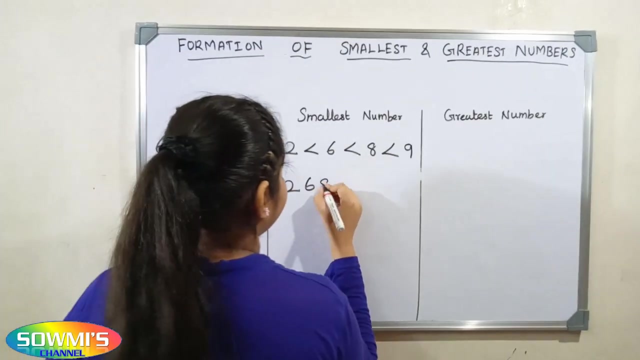 to largest number. Here, the smallest digit is 2.. 2 is less than 6.. 6 is less than 8.. And the largest digit is 9.. 3 dominating. 1,, 2,, 6,, 9400 are uppercase. The smallest wnumber formed by these digits is: 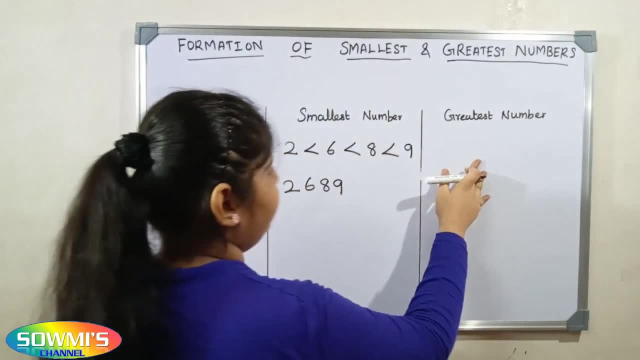 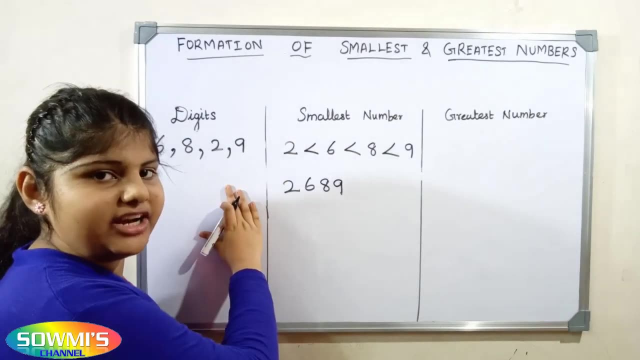 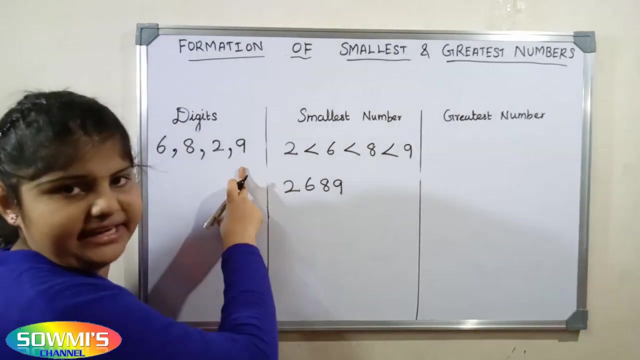 2689.. So the smallest number formed by these digits is 2689.. Next we will see how to form greatest number. To form greatest number, we have to arrange these digits from largest number to smallest number. Here the largest digit is 9,. 9 is. 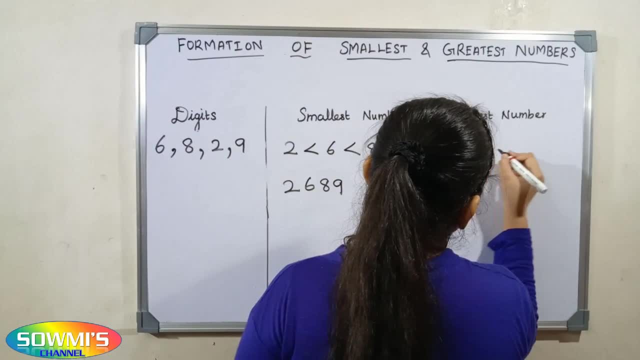 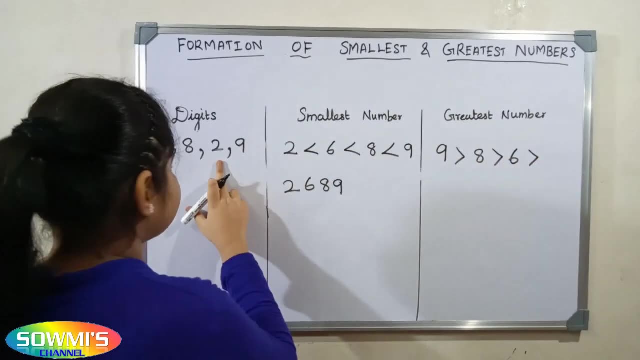 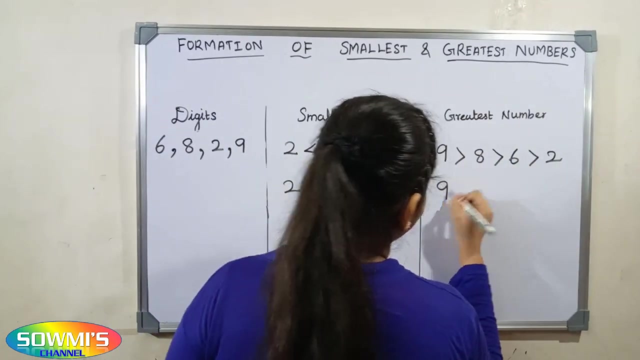 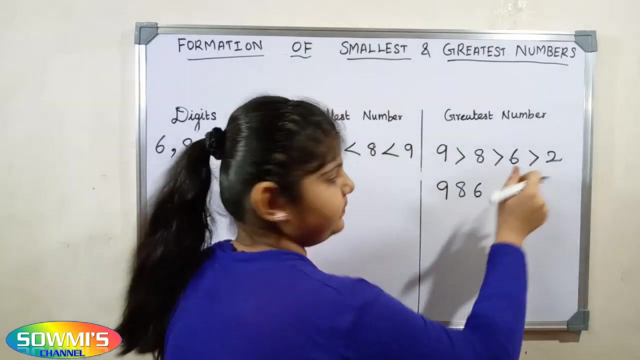 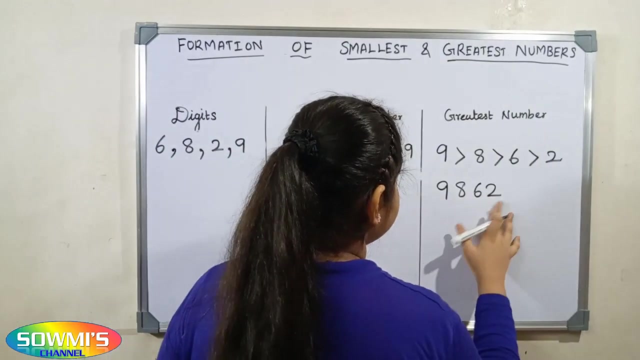 greater than 8,, 8 is greater than 6, and here the smallest digit is 2.. So the greatest number is 9, 8, 6, 2.. The greatest number formed by these digits is 9862.. Next we will take another example. 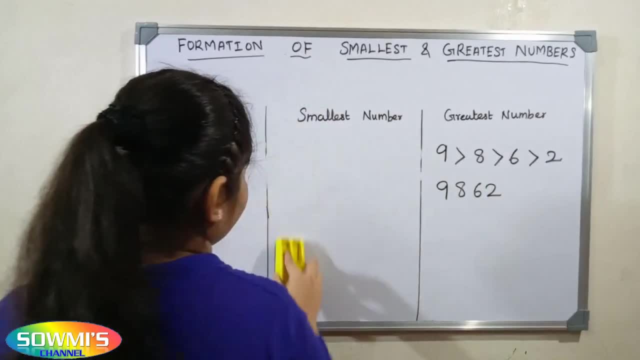 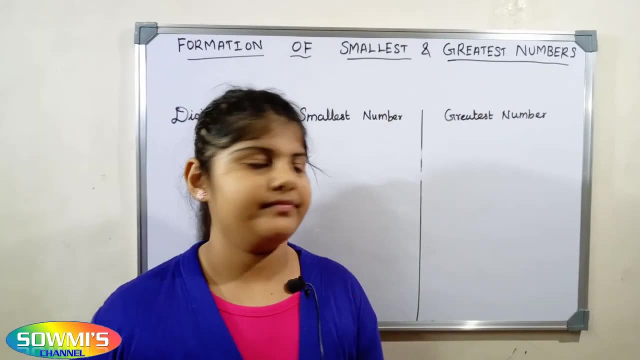 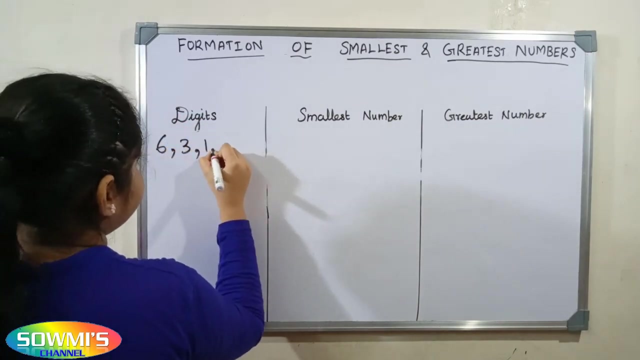 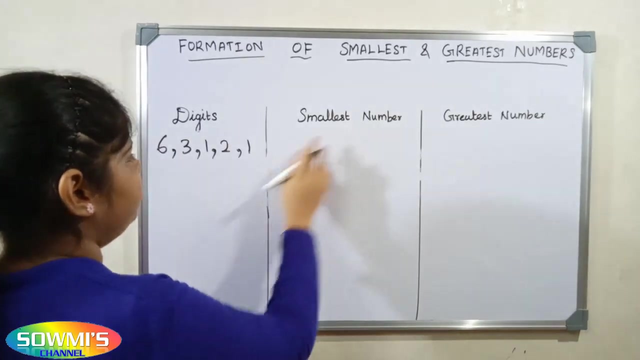 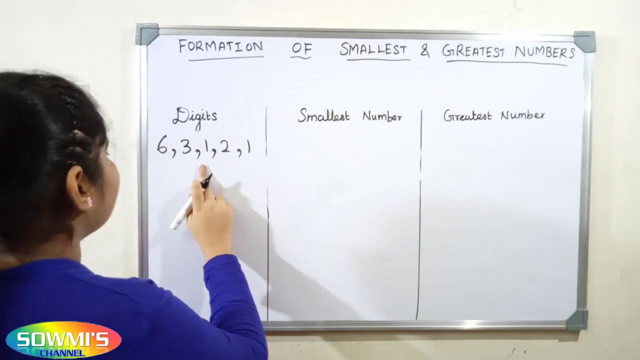 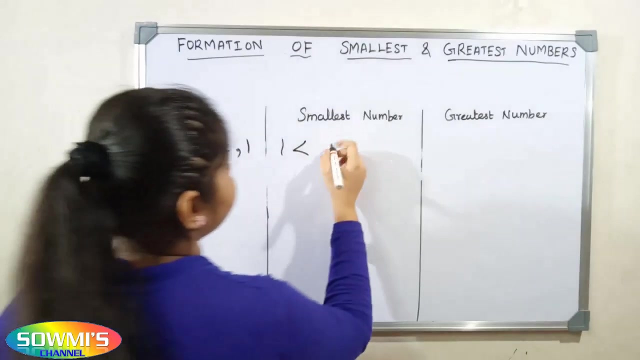 For example, we can take 6, 3,, 1,, 2 and 1.. First we will form smallest number. To form smallest number, we have to arrange these digits in a statement order. Here the smallest digit is 1.. 1 is less than 2.. 2 is less than 3.. And here the 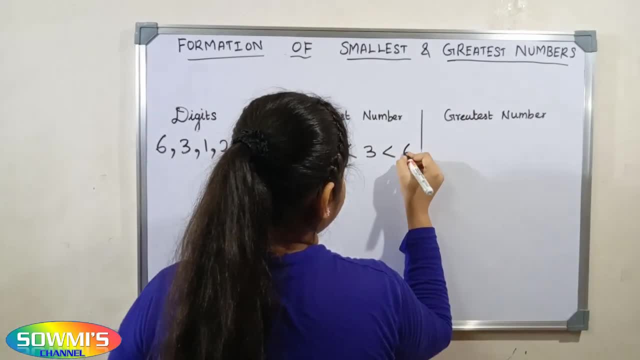 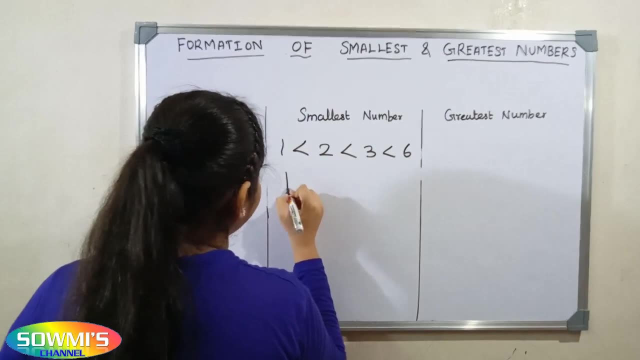 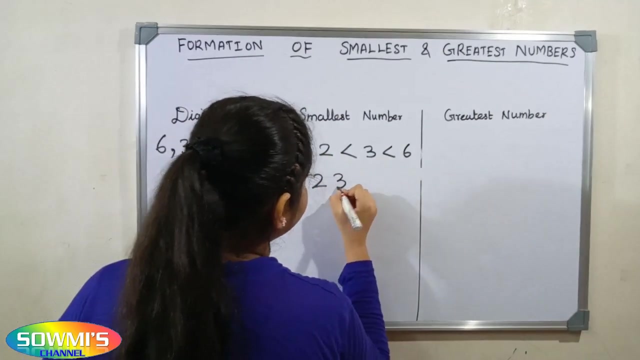 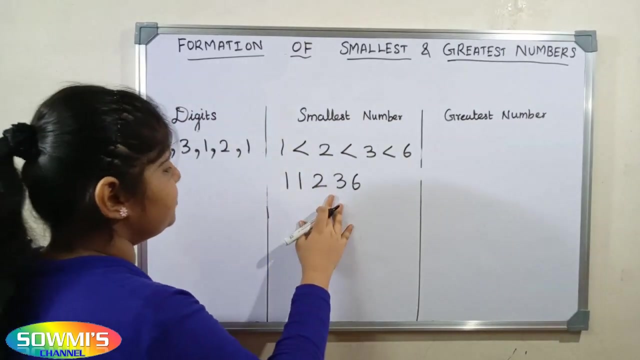 largest digit is 6.. Here 1 is repeated, So the smallest number is 1, 1,, 2,, 3,, 6.. The smallest number formed by these digits is 11,236.. Next we will see how to form greatest. 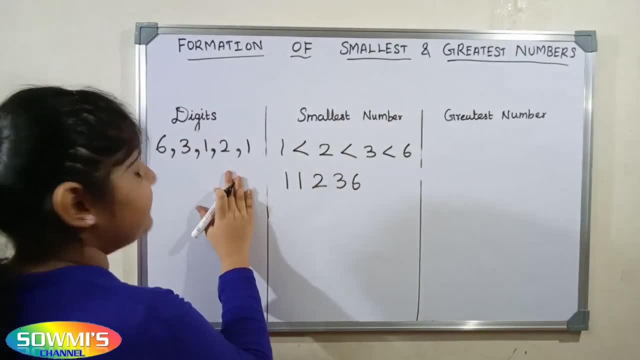 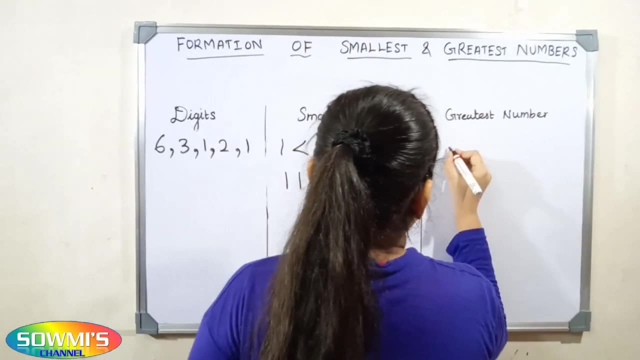 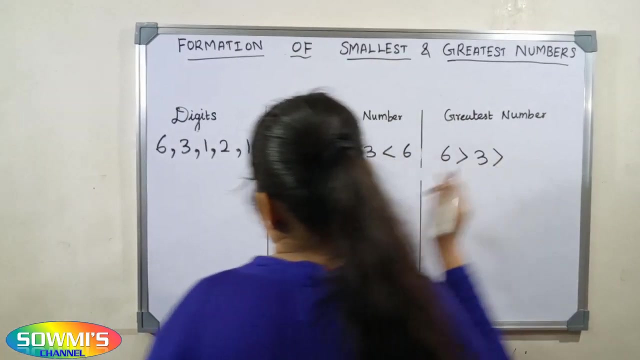 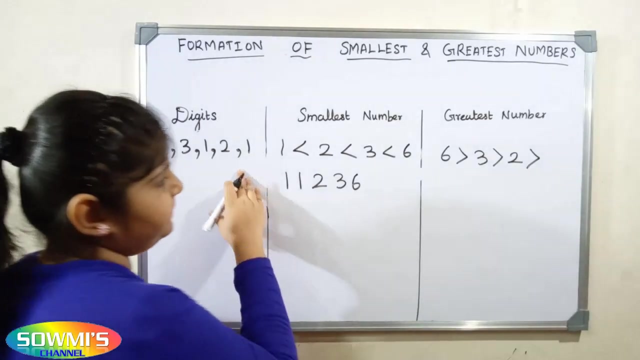 number To form greatest number. we have to arrange these digits in descending order. Here the greatest digit is 6.. 6 is greater than 3.. 3 is greater than 2.. And here the smallest digit is 1.. Here 1 is repeated, So the greatest number is 1, 1,, 2,, 3,, 6.. And here the smallest. 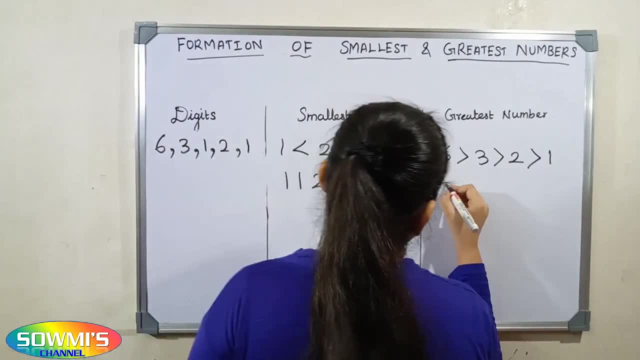 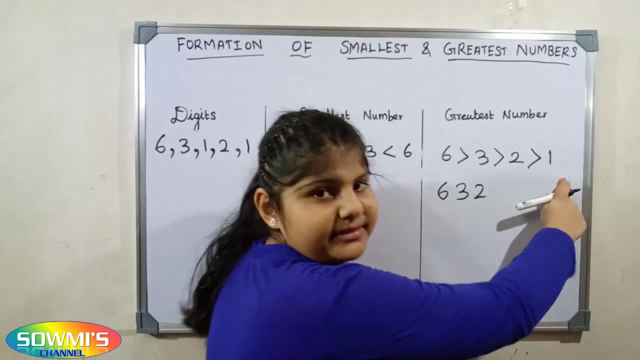 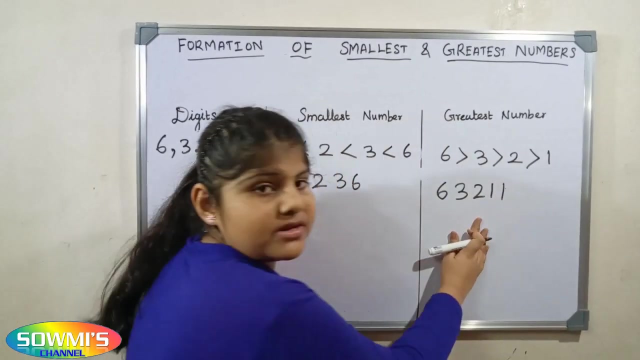 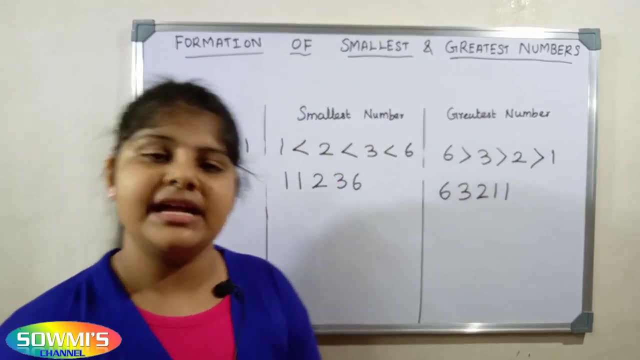 digit is 1, 1,, 2,, 1, and here is the greatest number. Here 1 of them is greater than 1.. Next we will see how to form greatest number. Here, 1 of them is greater than 3,, 3,, 6,, 6, and. 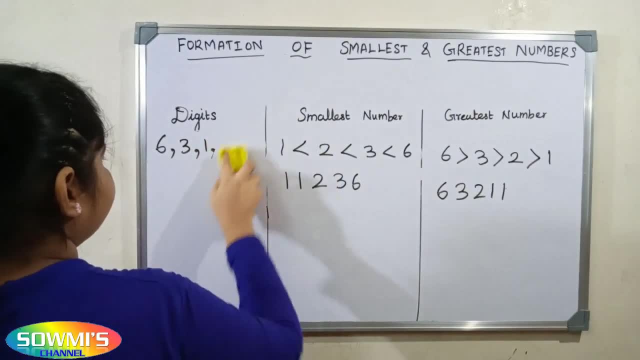 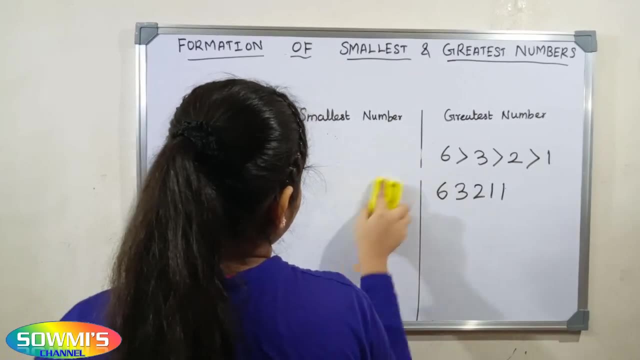 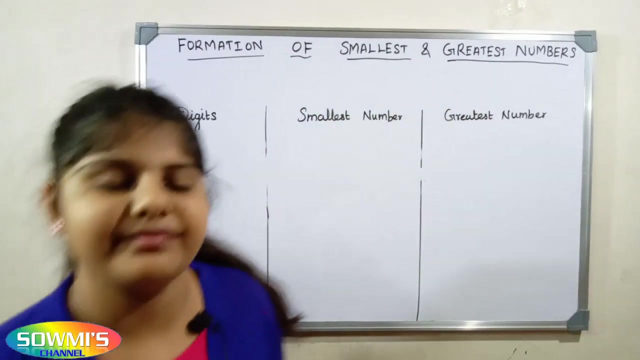 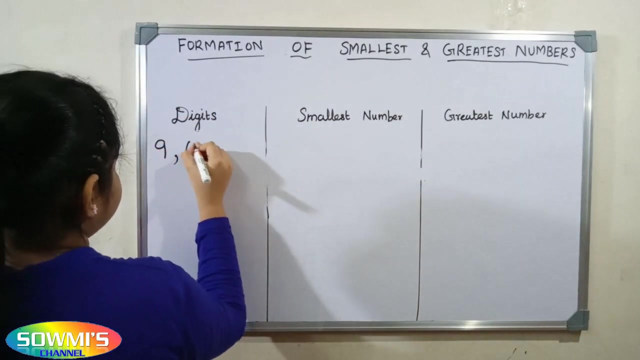 here this 1 is a greater number, So the greatest number formed by these digits is 63,211.. Next we will see how to form of greater than, or greater than or greater than 2.. So the greatest, For example, we can take 9,, 0,, 2,, 7..